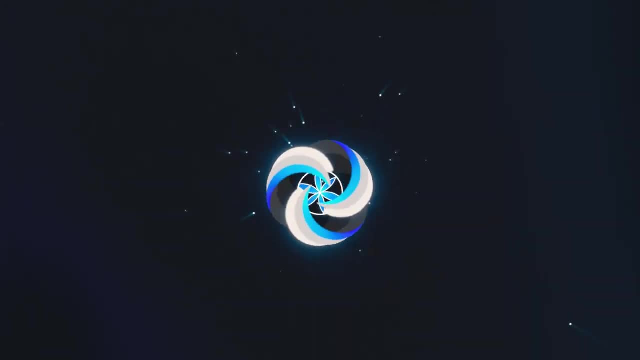 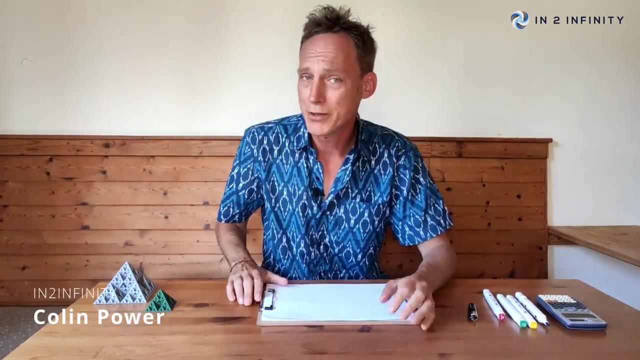 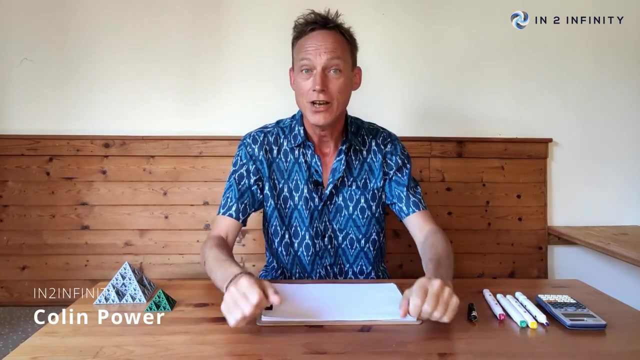 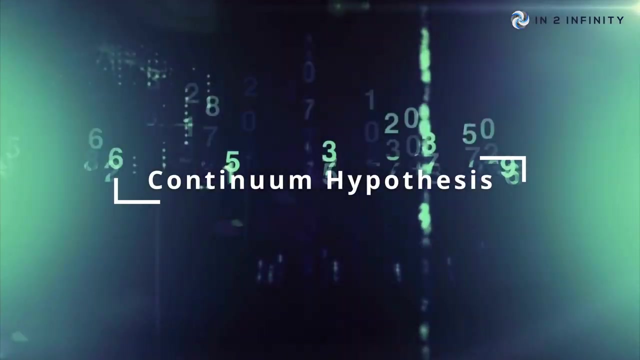 My name's Colin Power from Into Infinity, and today we're going to be solving the world's most challenging problem of the last century- the Continuum Hypothesis- using just a piece of paper and a pen. Before we do, let's have a little think about this nature of infinity. It started to become. 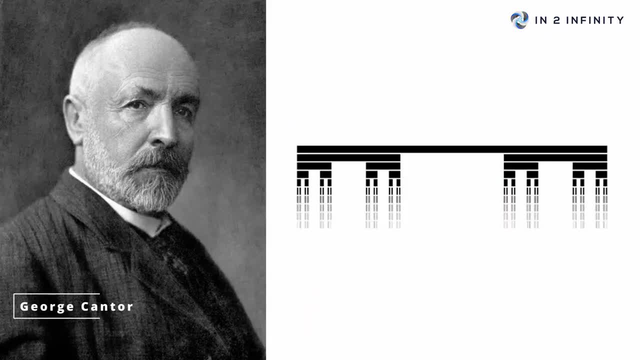 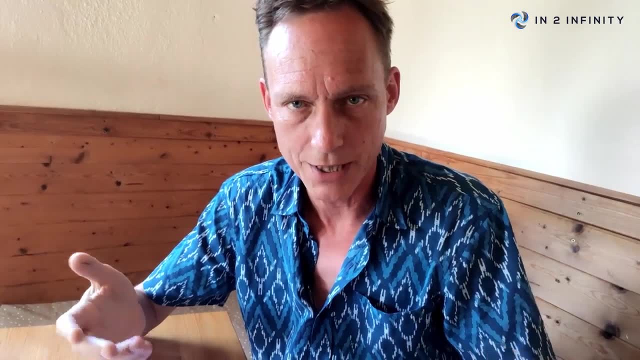 quite a topic at the end of the 1900s, when a guy called George Cantor described something called an infinite set and started to differentiate between different types of infinity. So here we have a line and it's divided into three. And what George Cantor did? he said what. 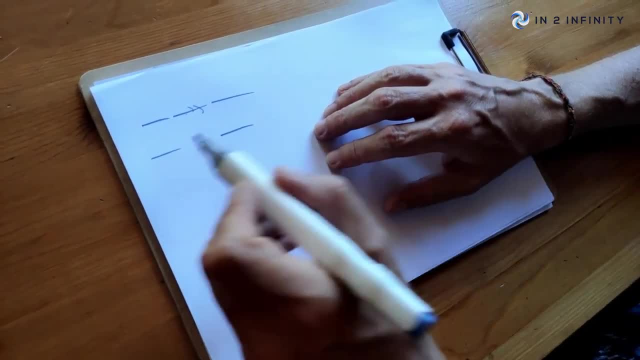 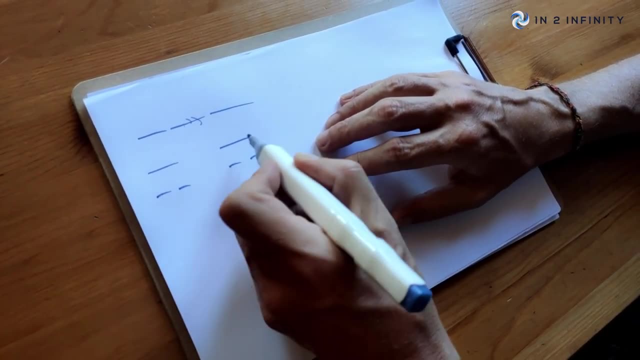 happens. if we remove that line, You'd be left with just two, So one third would be missing. And then, if you could, you can, you can also divide that and take out the middle Third of these parts and another third missing there, third missing from there, And each. 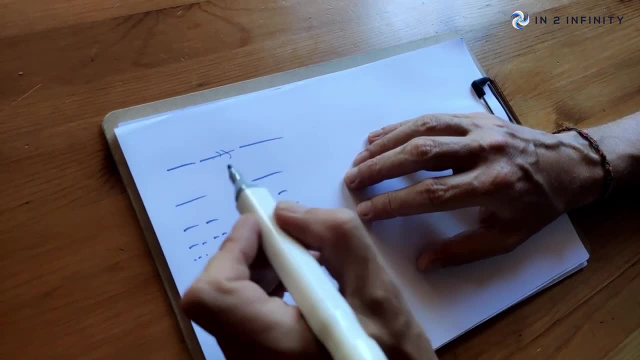 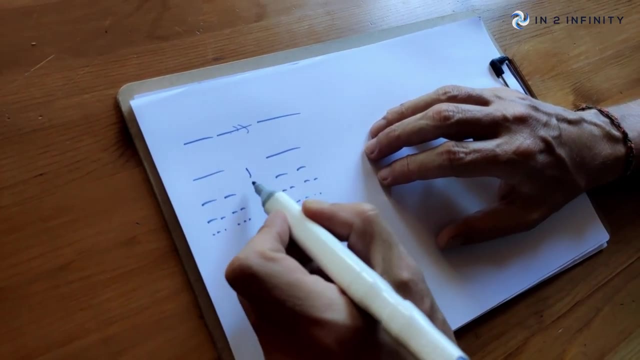 time we move through, we're removing a third section from the middle of each line, And so you can continue moving a third into infinity. Yeah, So the gap here. there's an infinite number of those gaps that you can create. Yeah, Those gaps there, There are also an. 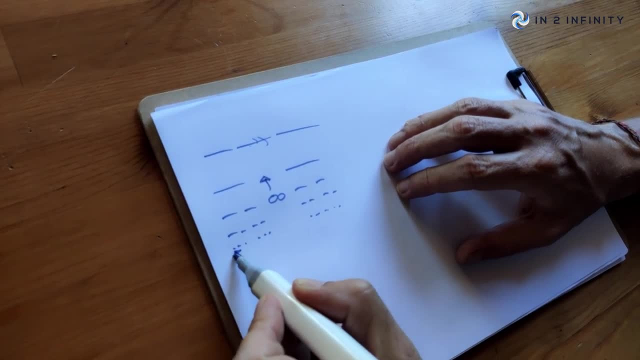 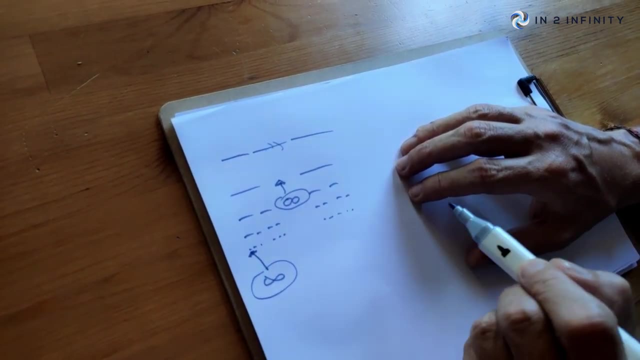 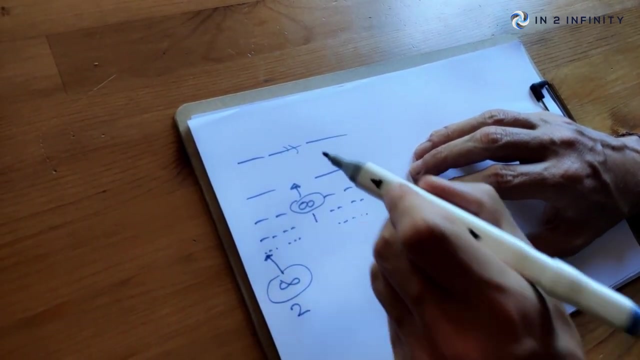 infinite number of these things here, But if you think about it- because there's two of those- that this is a larger type of infinity And this infinity here, this infinity, has one, two for every one that's missing there. So that's two for every one there. So that shows you that there are different types of 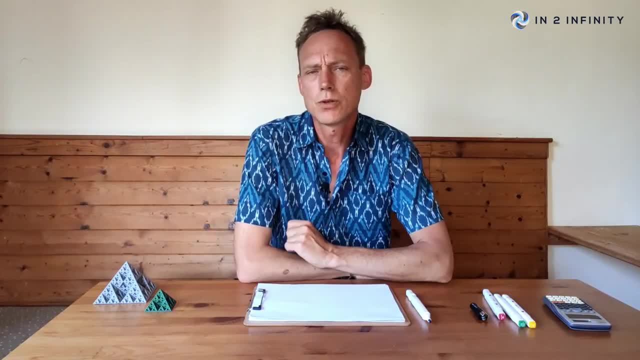 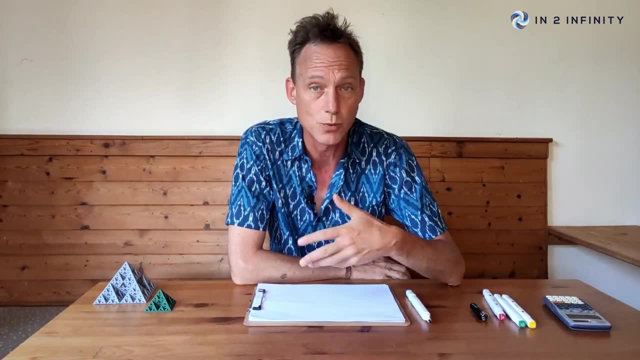 infinity. It was the birth of something called fractal geometry. This caused a little bit of a stir in the mathematical community, you could say, but it did lead to something which is the foundations of modern mathematics, called set theory. And so the concept is that we 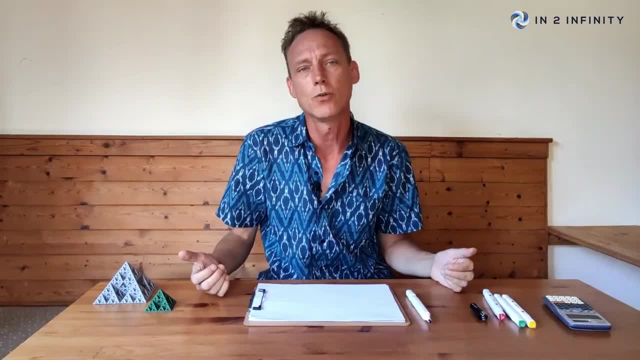 can have different types of set. So, for example, let's take all of the numbers one, two, three, four, five, six, seven, eight, nine, 10,, 11,, 12,, 13,, 14,, 15,, 16,, 17,, 18,, 19,, 20,, 21,, 22,, 23,. 24,, 25,, 26,, 27,, 28,, 29,, 30,, 30,, 31,, 24,, 35,, 38,, 39,, 40,, 41,, 42,, 42,, 43,, 44,, 45,, 44.. 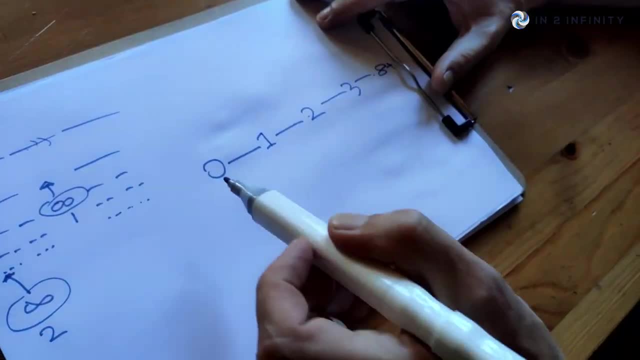 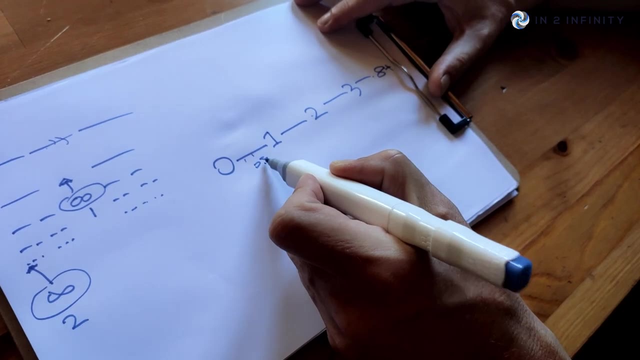 On into infinity. We could say that is a certain set of number, But the problem is is, as we go through these numbers, there's a lot more numbers in between here. Look, that would be naught: 0.5,, for example, yeah, Or 2.5, yeah, wouldn't it there? And actually there's. 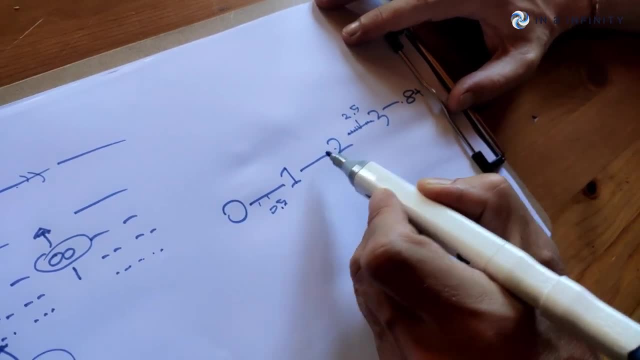 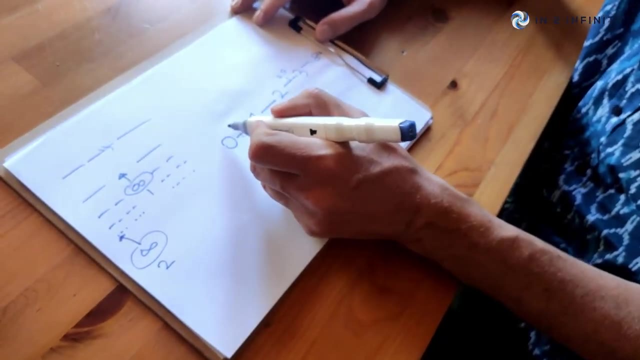 an infinite number of these tiny little divisions in between each number space, And that creates a sort of bit of a conundrum, really, Because in this sense we could say that this is one set of numbers and that set of numbers is an infinite set. 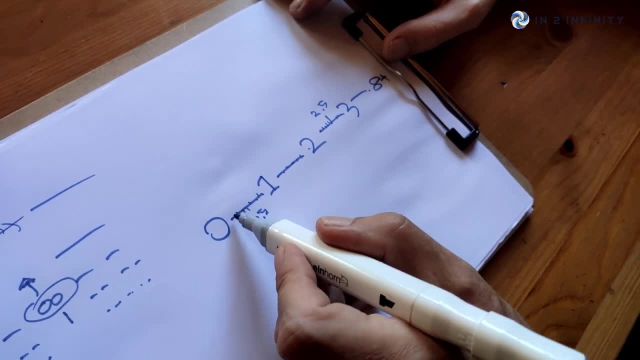 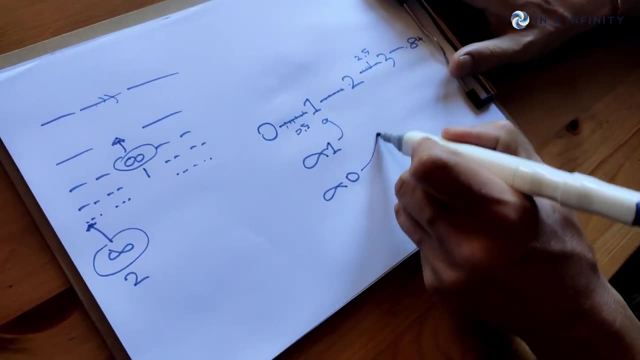 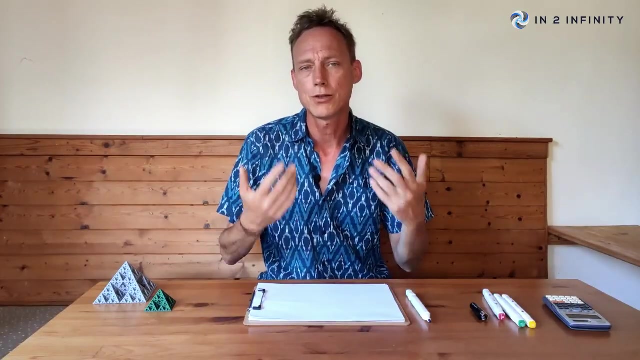 but it's smaller than this which they call, you know, the infinite set of real numbers and everything else like that. yeah, lf1 is all of these whole numbers and lf0 is including all of all of that set, including all of those small numbers. you know, to solve the continuum hypothesis cantor suggested: 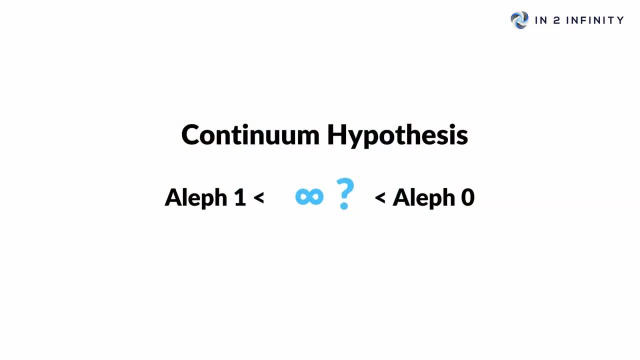 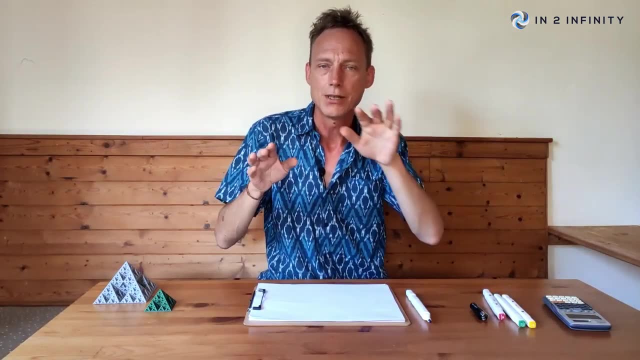 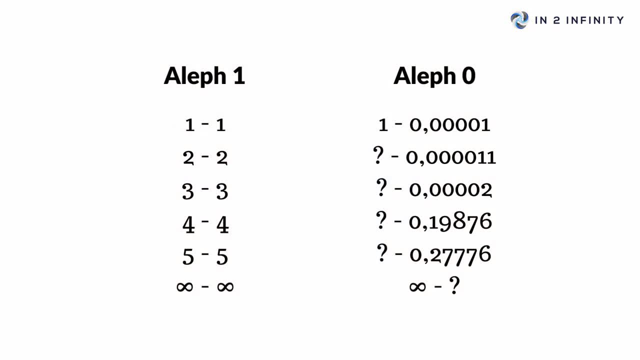 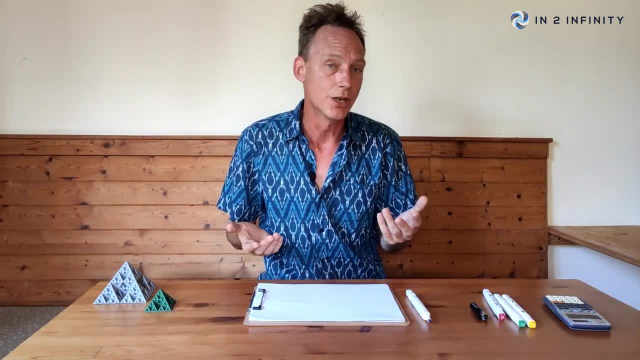 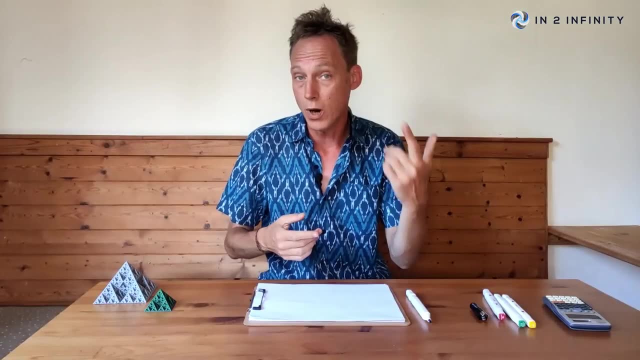 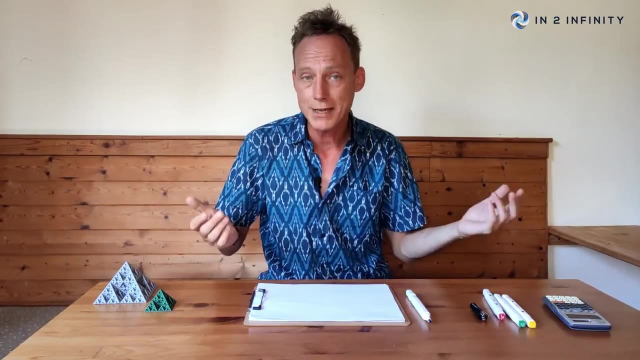 with a zero point and because of that nature it creates a paradox in mathematics. you can imagine: lf1 would be the whole numbers one, two, three, four, five, six, seven, eight, nine, ten into infinity, whereas alat0 would include all of the decimal fractions as well. is there an infinity between? 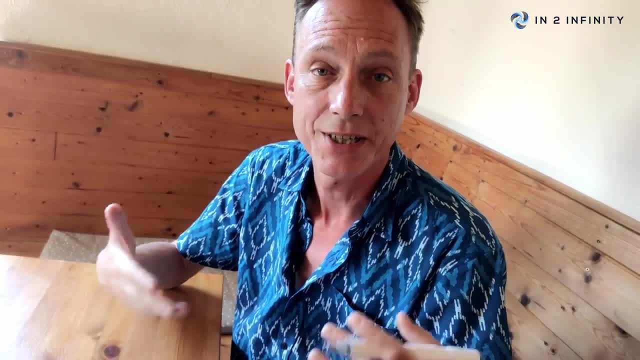 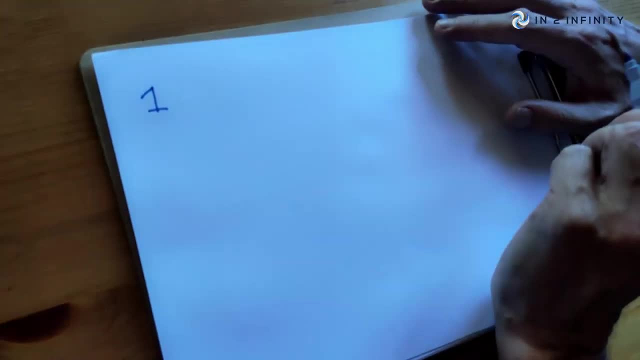 lf1 and lf0, and we're going to prove that there is actually an infinity between lf1 and an f0. so, to start with, we've got a column over here. we write the number one in there. yeah, that's our step one. and over here, what we're going to do is we're going to write 1 over 1. it's a fraction, yeah. 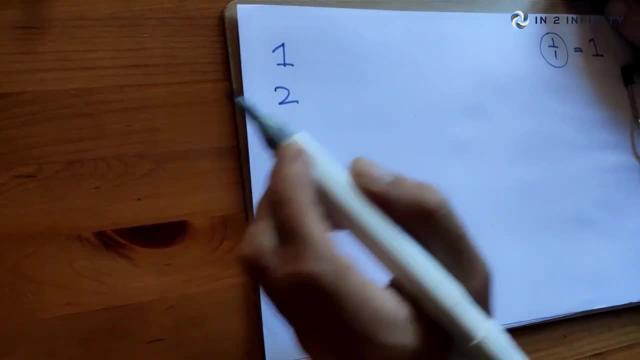 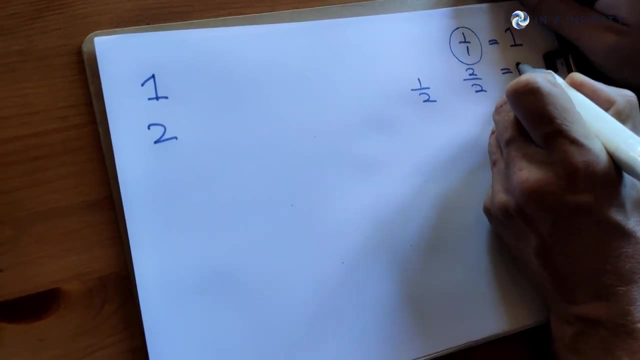 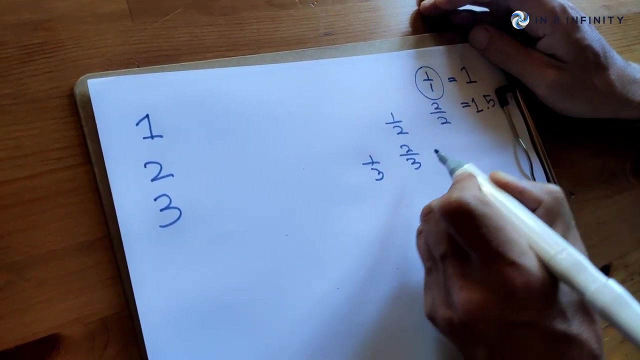 1 over 1 equals 1.. so let's go to the second step. yeah, and here we're going to go 1 over 2, and then 2 over 2 equals 1.5, and as we go to number 3, we're going to get 1 over 3, 2 over 3 and 3 over 3, like that and that. 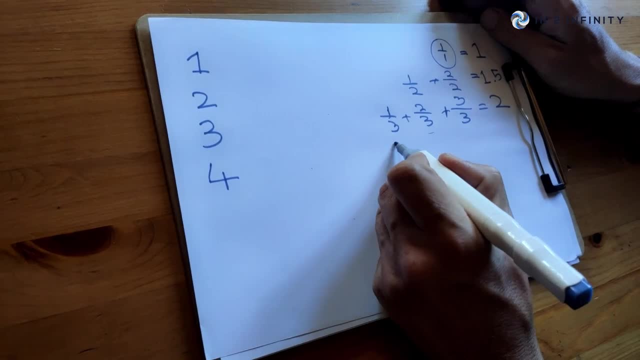 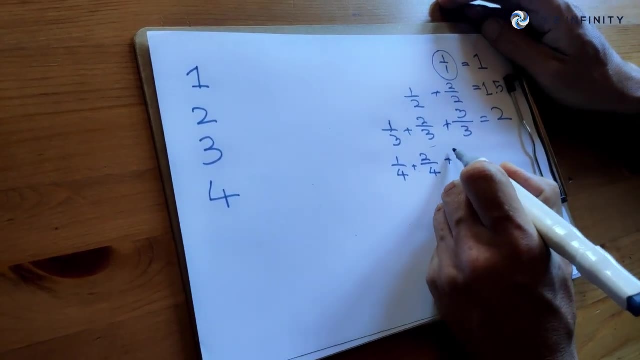 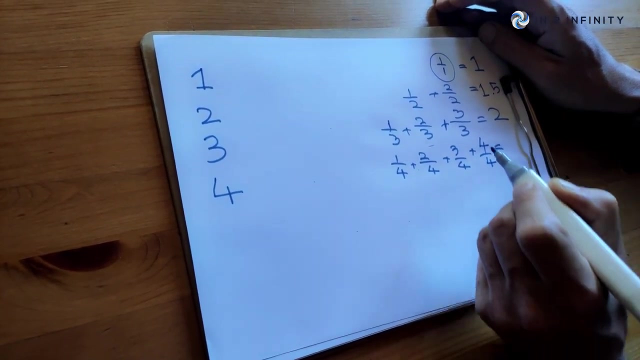 equals 2, and I'll go to the fourth step just to show you: 1 over 4, 2 over 4, the plus sign there, plus 3 over 4, plus 4 over 4 equals 2.5 and you can see what's. 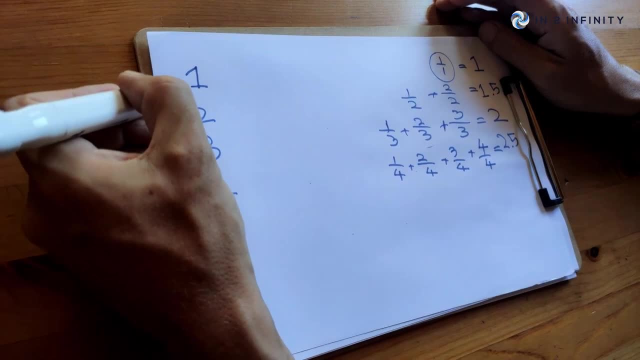 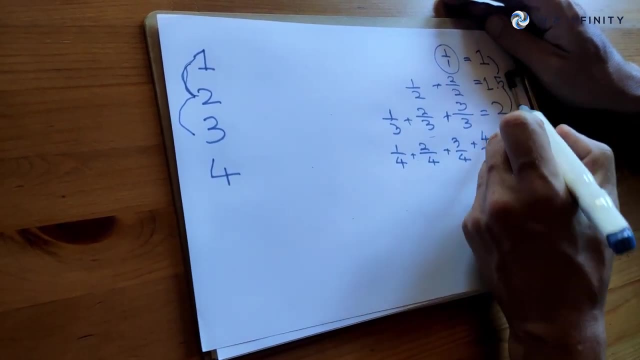 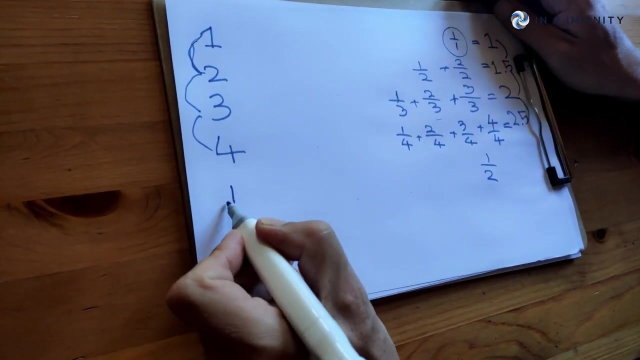 happening here is that every step this takes a one step, goes one and jumps down there. when this jumps down, it jumps down just a half, and this jumps down to one, this jumps another half, this jumps to one, this jumps another half, and so this takes a half which is progressing at one. yeah, and it will continue like that. 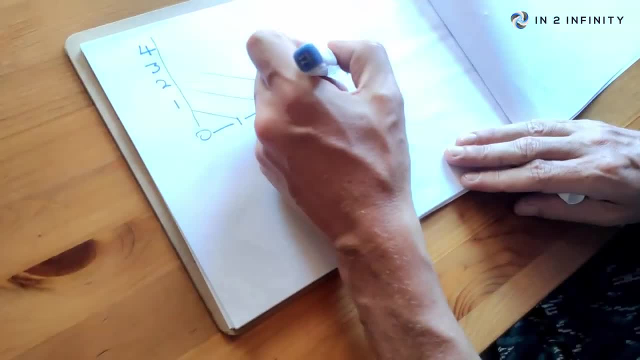 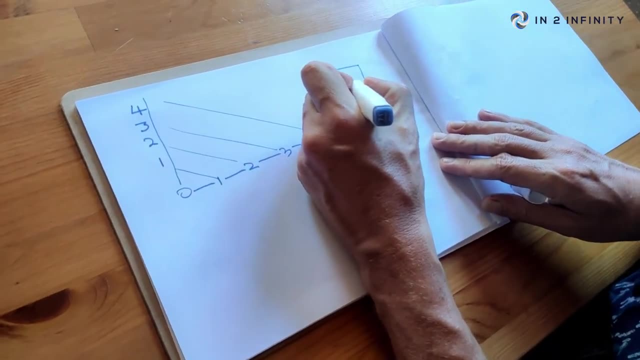 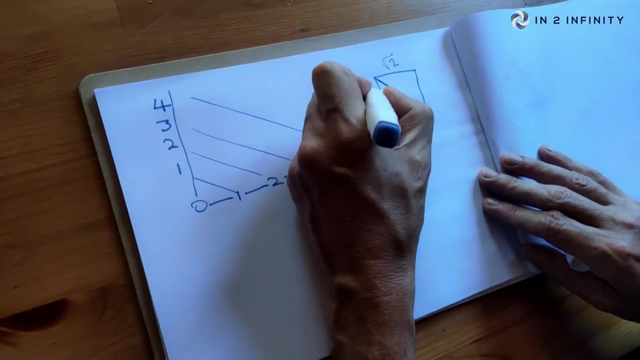 on into infinity, and so each one of these lines connects along like that, and really what you get is, if you think about it, you get a square like that, with a diagonal being straight the way through, yeah, which- and we call that the square root of two, yeah, if we call that a unit of one, yeah, so that's a square. 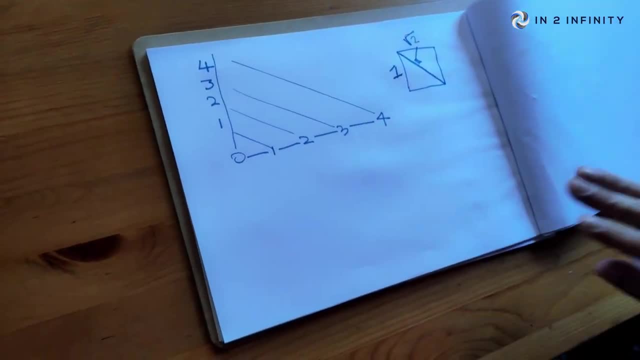 root of two going across that middle line there. yeah, now if we take LF 0.5, because of the square root of two, we're going to have a square root of two and because it's only progressing in half steps, and so actually it goes up like: 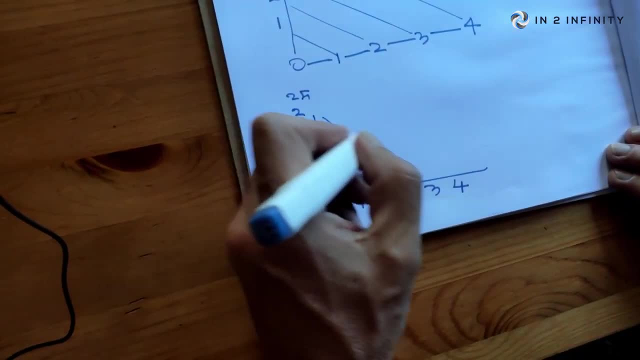 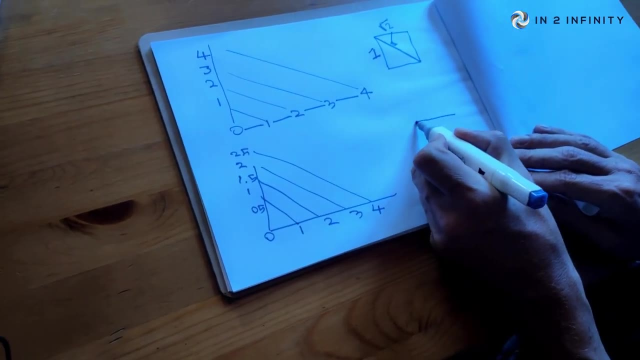 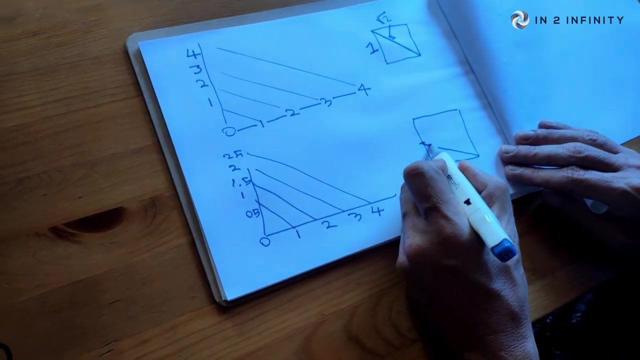 this and it goes from one to one one to one point, five point, another point like that. but because this is, this is shrinking, yeah, in size, it's only stepping up in half. what you would get is if we turn it into a square again, this would be the halfway mark, and this would go like that, and that would be the. 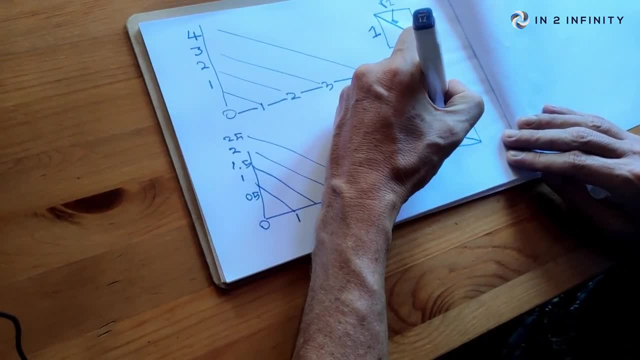 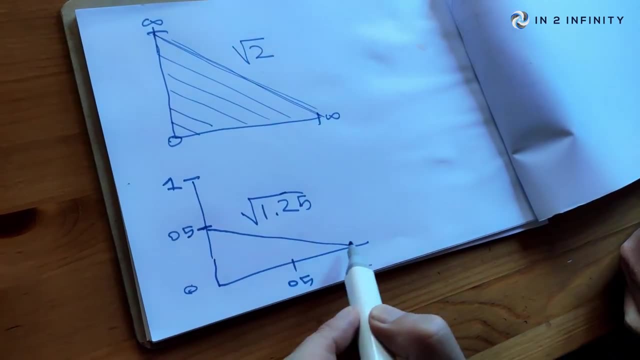 geometry of that, and then this here would become the square root of 1.25. but you can see here that there's a geometric nature to this type of infinity, that this infinity is denser because it's compressed, and that means we can compress things to the halfway mark. the 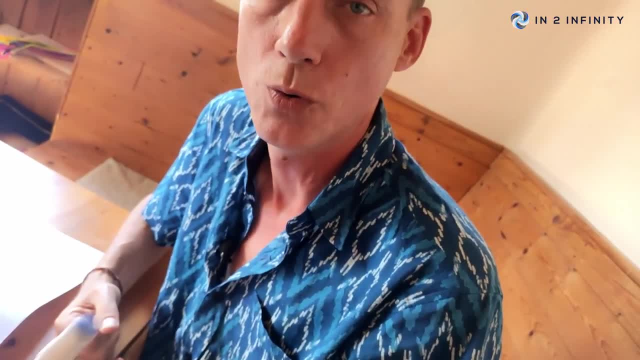 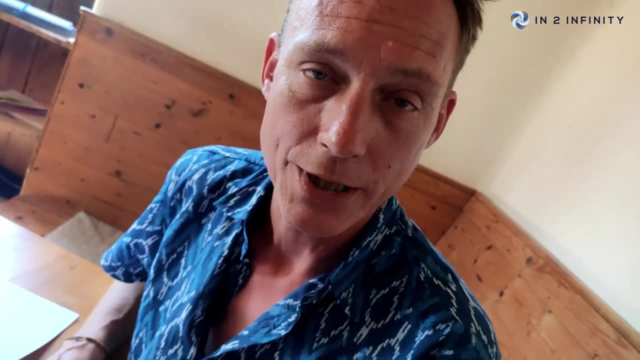 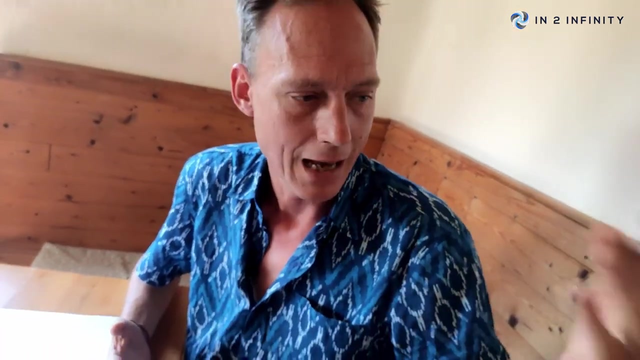 0.5 mark and that's why we call it LF 0.5. so that's resolved, the continuum hypothesis. the question was: is there an infinity? that is, you know, falls in that straight line between, you know, the LF 0 to the infinity of all numbers, to LF 1, which is 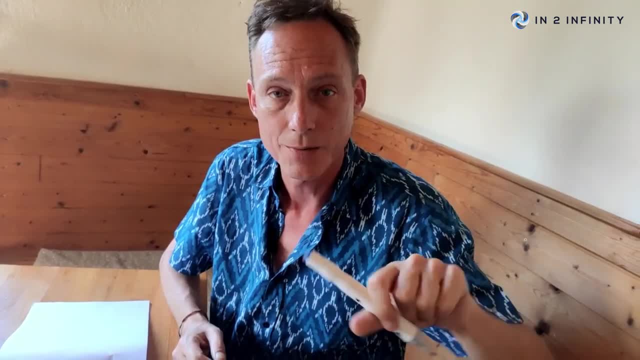 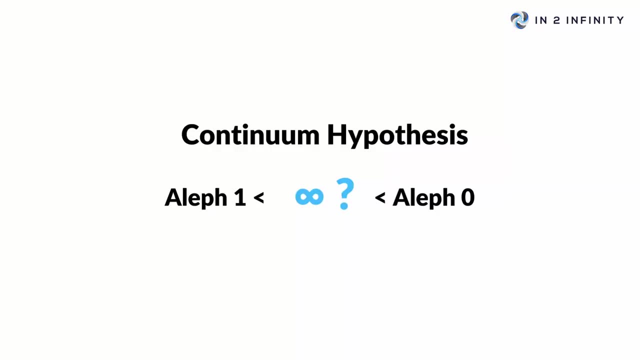 the infinity of the whole number set and there is an infinity between the two and it's the fractional numbers between 0 and 1, and that proves that George Cantor's conjection that there isn't an infinity between these two wrong. and there is actually one, and it's called LF 0.5. and now LF 0.5 has many. 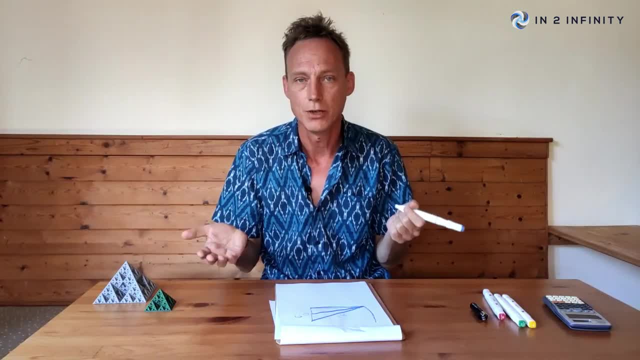 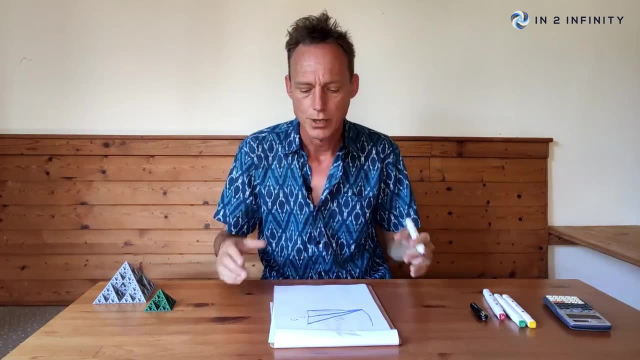 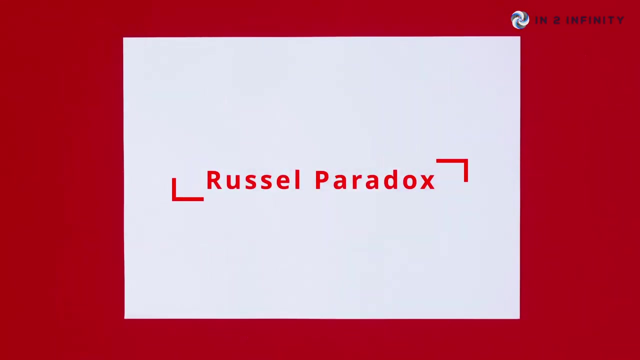 implications for a lot of other things in mathematics that we're going to look into next, yeah, but before we do, we're going to also maybe give a bit more of a satisfying solution to what this kind of means for numbers and infinite set theory. so coming up next, yeah, will be a solution to the Russell paradox, and 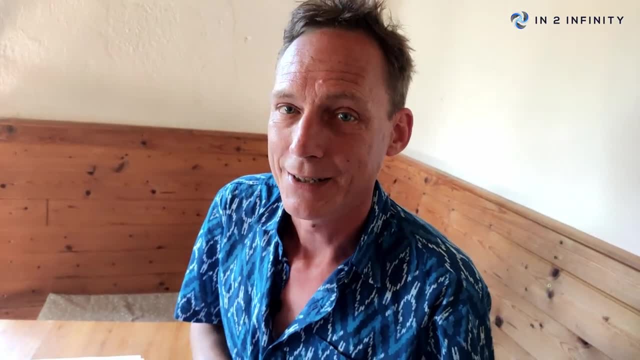 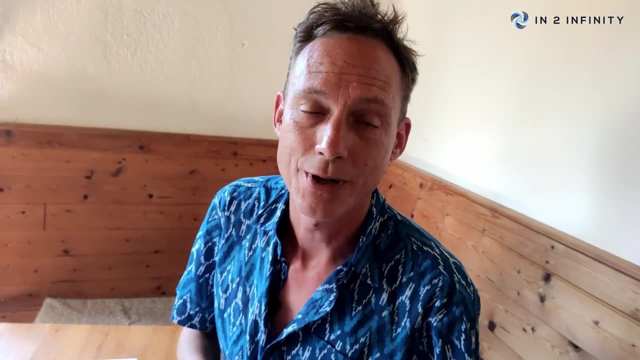 much, much more. so remember to subscribe below and if you want to follow along with us and if you like what you see, do subscribe to our patreon and where you can get access to webinars and taught us more about all this sort of stuff directly. thank you very much. my name's been Colin Power. you've been awesome. 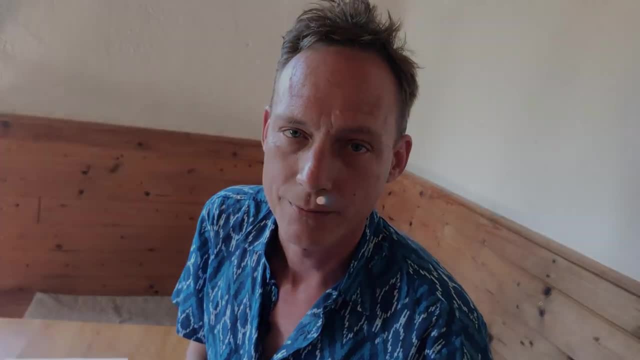 this is into infinity, taking you beyond the matrix. you. 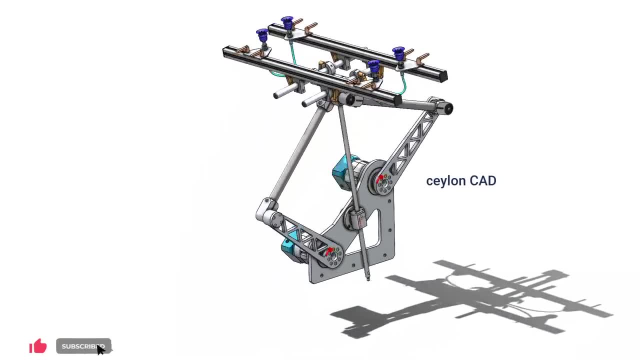 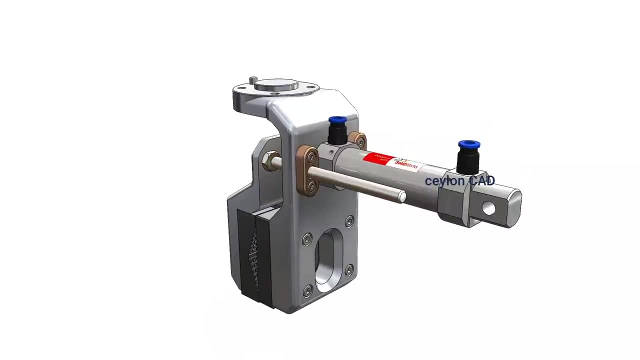 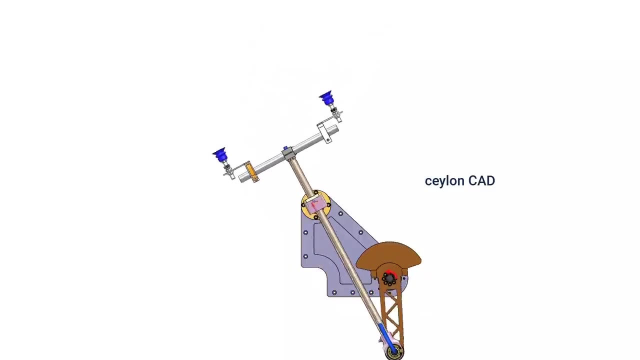 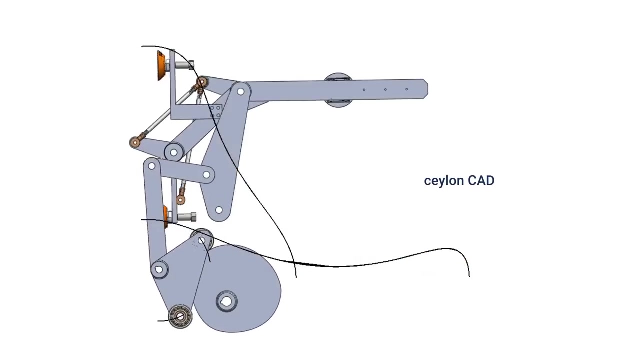 Prepare a paper with an eye and an eye. Take a card, Draw a line, Cut the line. Take a card. Draw a line, Cut the line, Draw a line. Take a card. Take a card, Draw a line. You're giving me wind and rain.